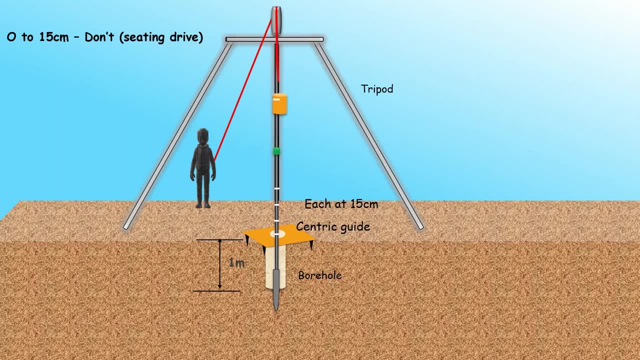 Now drop the hammer through 75 centimeter height and start penetrating the soil. Did you start counting the blows? Now you should not Here. blows required for first 15 centimeter penetration is not considered as it is a sitting drive. Blows required for second and third 15 centimeter, that is, from 15 to 30 meters, is not allowed. 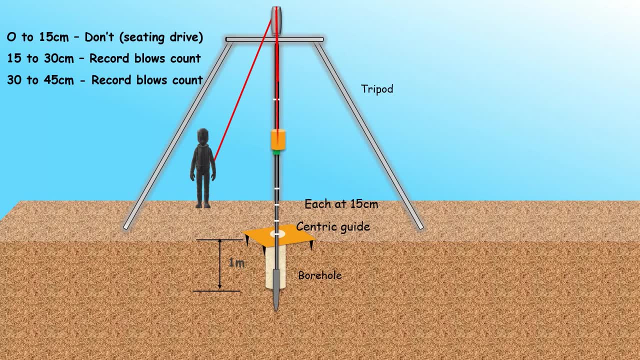 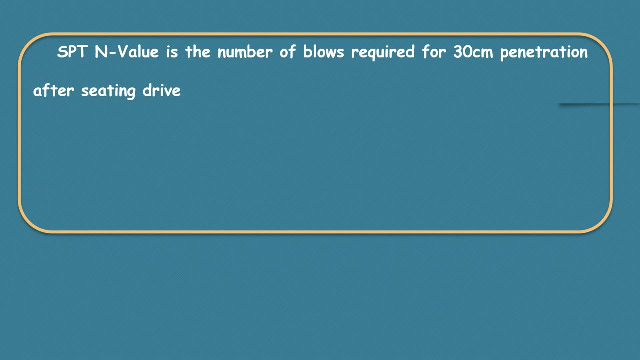 Highness of promo oils should not be considered unless even the price of the blower drop into 30 cm and from 30 to 45 cm is recorded and that gives n value recorded. So SPT n value is the number of blows required for 30 cm penetration after your seating tray. 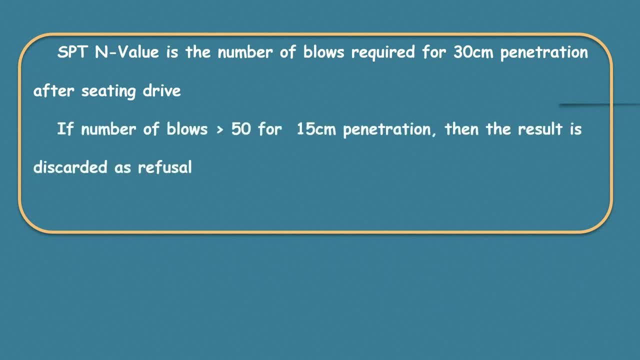 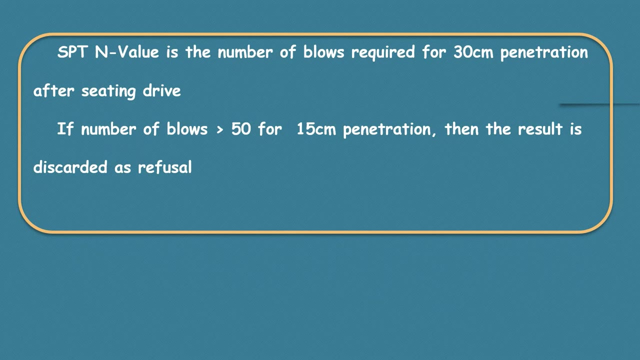 If number of blows are greater than 50 for a 15 cm penetration, then it is taken as ground refusal for your penetration. So don't consider that value. Your record and gain value has number of errors and hence it needs number of corrections too. 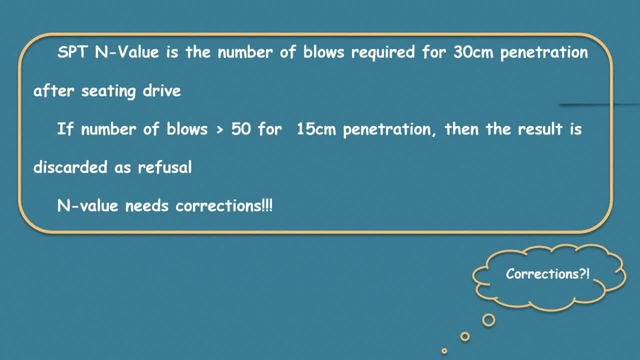 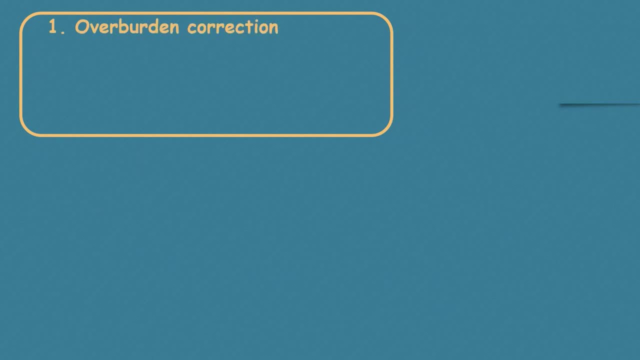 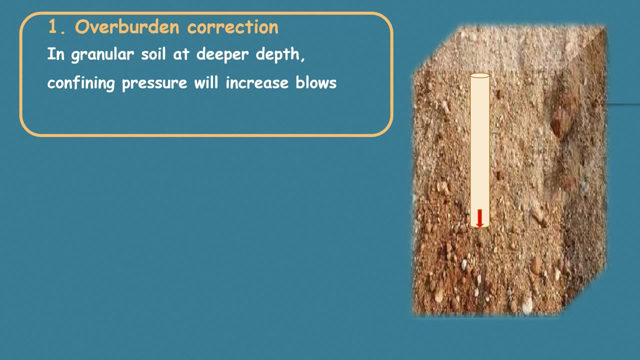 But IS code recommends two corrections in particular, Of which first one is overburden correction. In granular soil at deeper depth, confining pressure will increase. Hence we may overestimate the strata at deeper depth. IS 2131 recommends this graph for overburden correction. 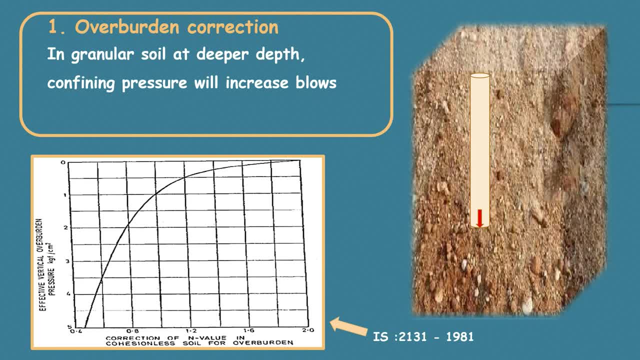 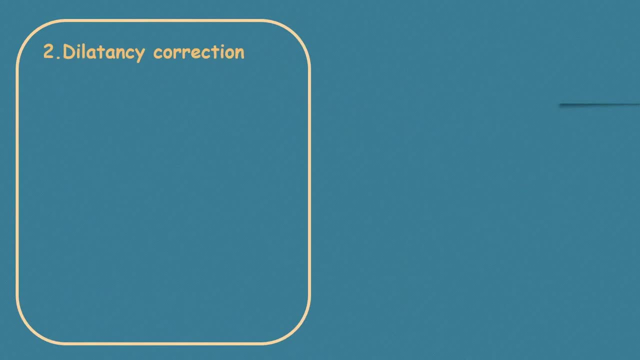 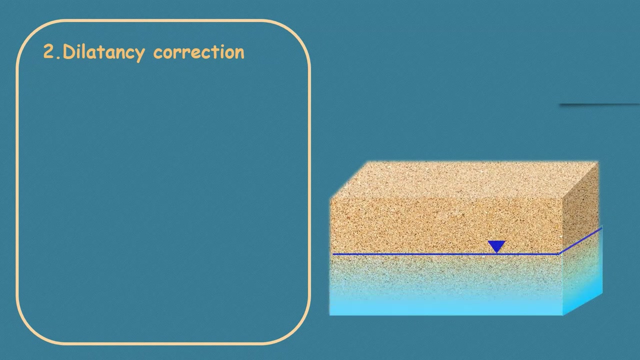 Apply overburden correction using this graph: Let the n value after applying correction be n0.. The next correction to be applied Is dilatancy correction If silty, fine Sand or fine sands are present below water table and n value after applying. 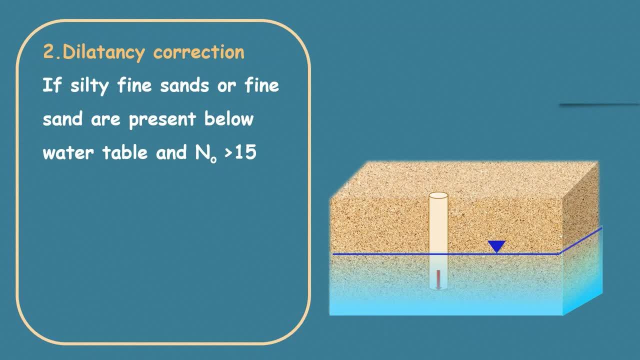 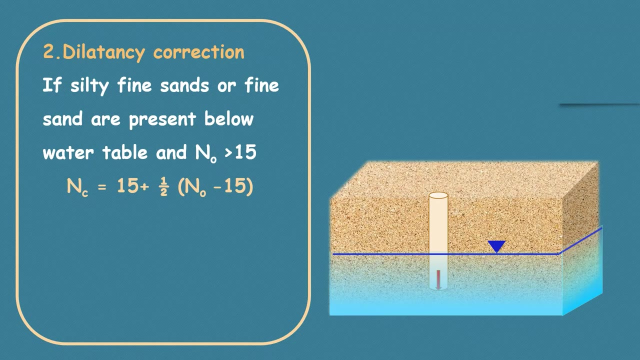 overburden correction is greater than 15, then the corrected n value is given, as Nc is equal to 15 plus half of n0 minus 15.. It is to be noted Here That overburden correction has to be applied first, and then the dilatancy correction is done.